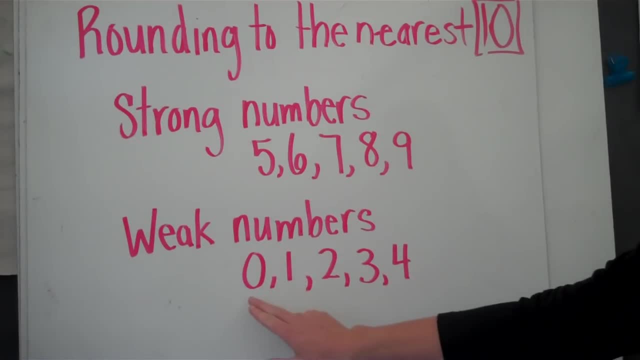 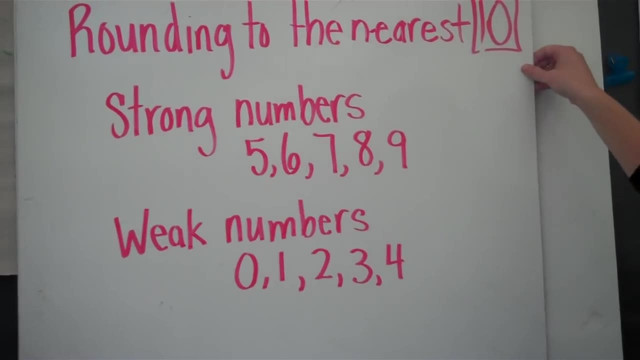 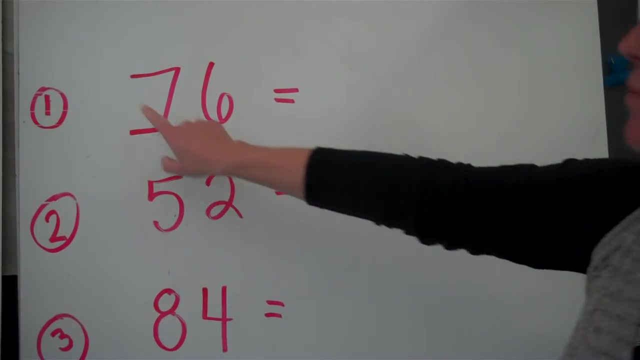 weak numbers, which means that the 10 doesn't change, are 0,, 1,, 2,, 3, 4.. Let's practice First. I know I'm rounding to the nearest 10, so I'm going to look at the 10's place. 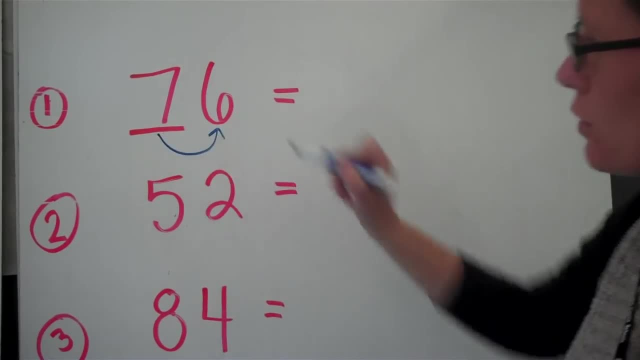 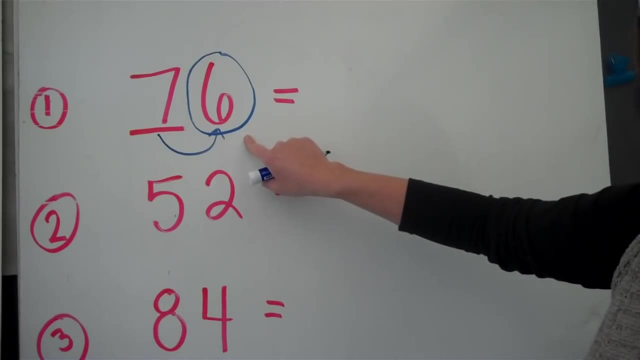 and I'm going to go one column over to the 1's. I'm going to circle my 1's and I'm going to go one column over to the 1's And I'm going to decide: is that number weak or strong? I know that the 6 is strong, which? 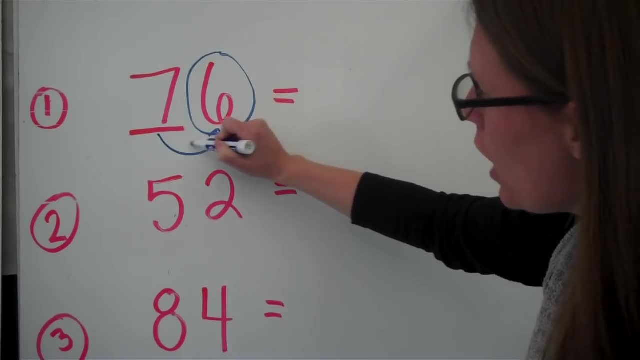 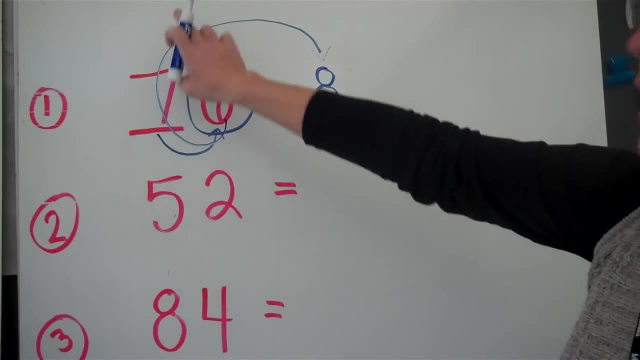 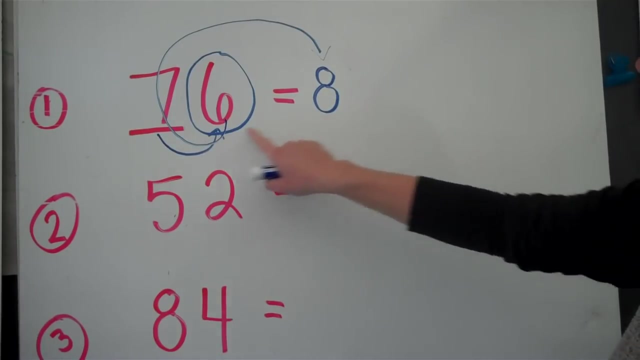 means it has lots of power. It's going to push up my 7 to an 8, because the next number I count up is 7, 8.. So my number is 8. And since I used all the power out of the 6,, the 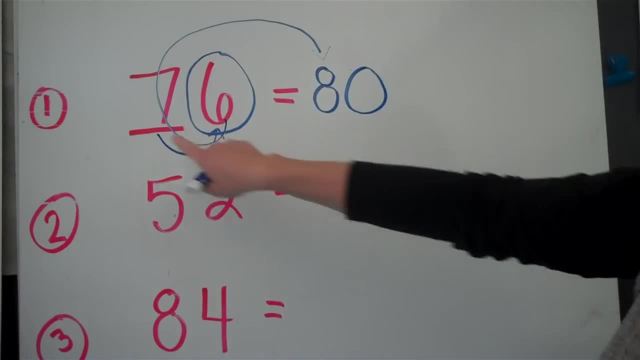 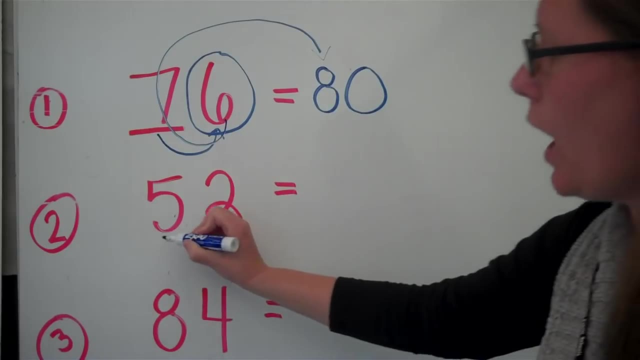 1's is 0. So my number is going to go up to the 6, and it's going to turn into a 0. 76 rounds to 80.. The next one, 52.. I know I'm rounding to the nearest 10, so I'm going to look one column. 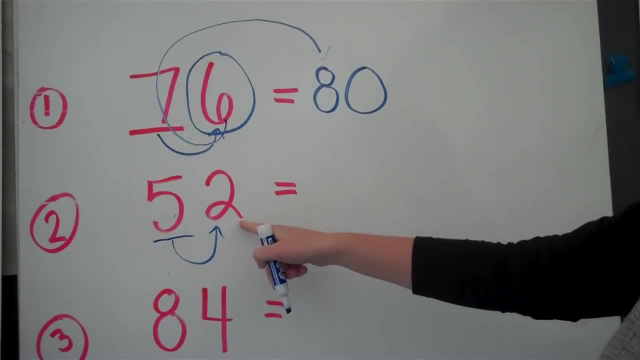 over to the right, which is my 2,, my 2.. I'm going to circle it, I'm going to decide: is that weak or strong? I know that 2 is weak. It has no power. So it's going to push up my 7,, 8,, 2,, 3,, 4.. And I'm going to go one column over to the 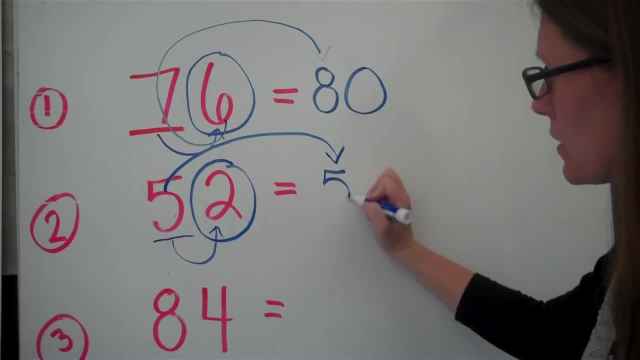 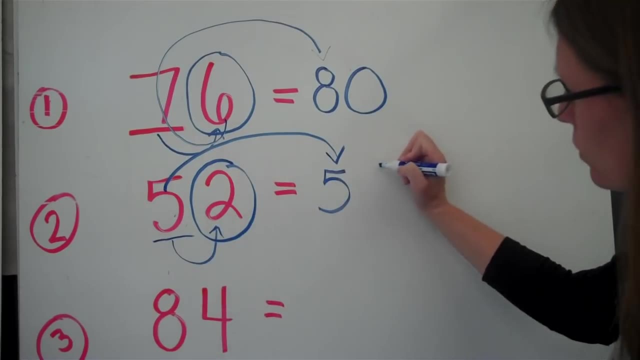 the five is going to stay the same, because two is weak, meaning that it has no power, It can't push it up, And the two is going to become a zero: 52 rounds to 50.. My last one, I know I'm. 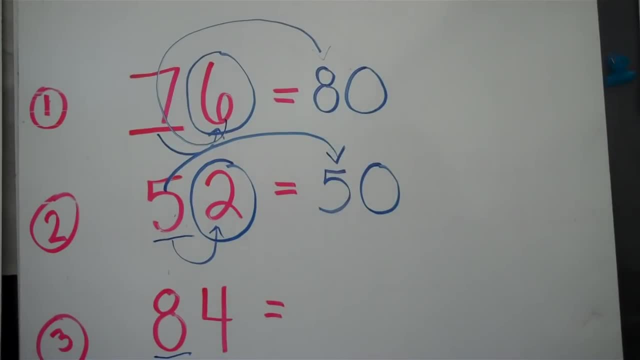 rounding to the nearest 10, so I put my line underneath my 10, go one column over. I have a four. Four is weak and has no power, so the eight stays an eight and the four turns into a zero. That should be a review. We are rounding to the nearest 10.. It gets a little trickier. 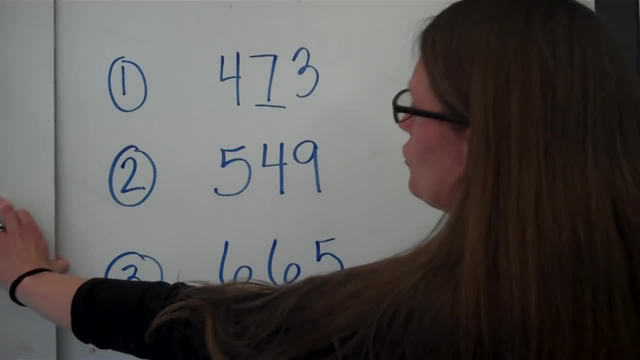 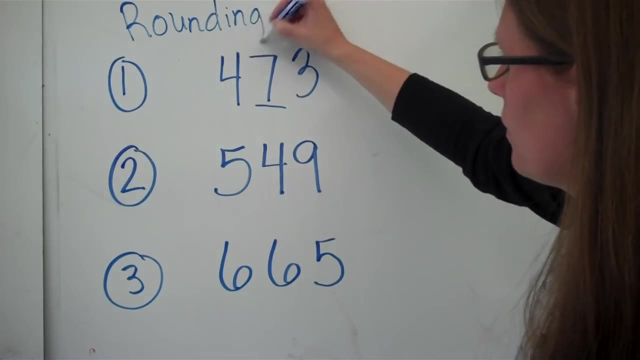 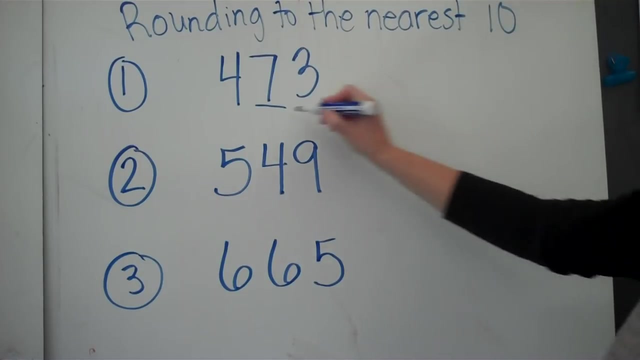 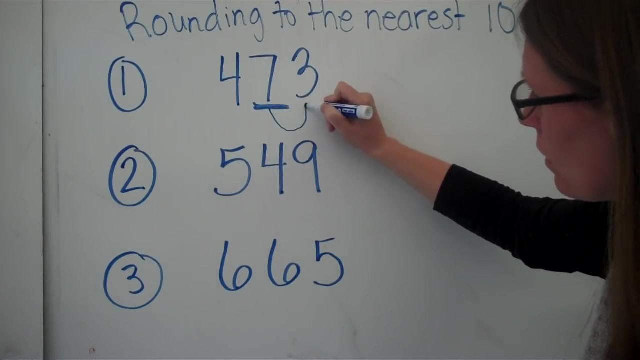 but not hard when you have hundreds and you are rounding to the nearest 10.. Okay, I'm still going to look at my 10's place. I don't care about the hundred right now. I'm going to move to the right. I'm looking at the ones. Is that number weak or strong? Three is: 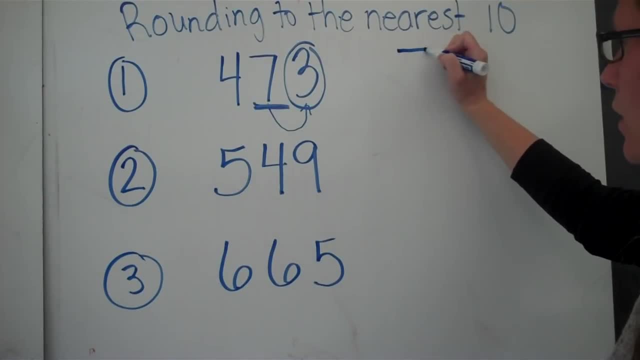 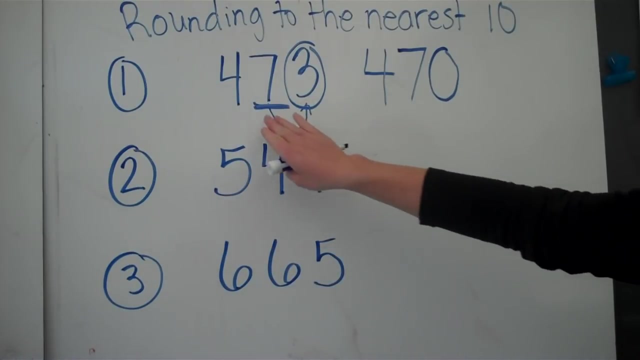 weak has no power to push the seventh, So I'm going to keep my seven in the 10's place. My three is going to become a zero and my four is going to stay exactly the same. I'm not looking at the hundreds today, I'm just looking at the tens. So 473 rounds to 470.. Let's look. 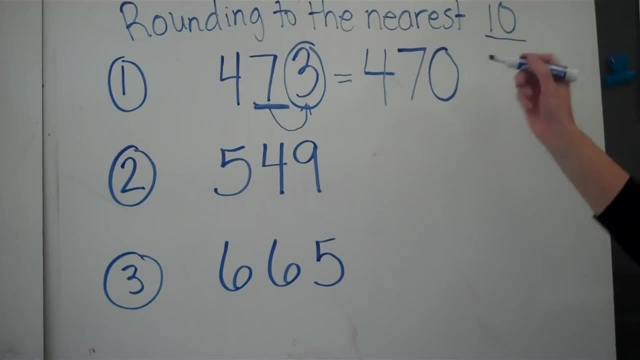 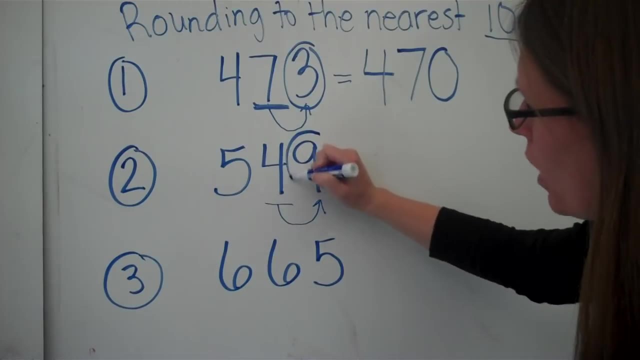 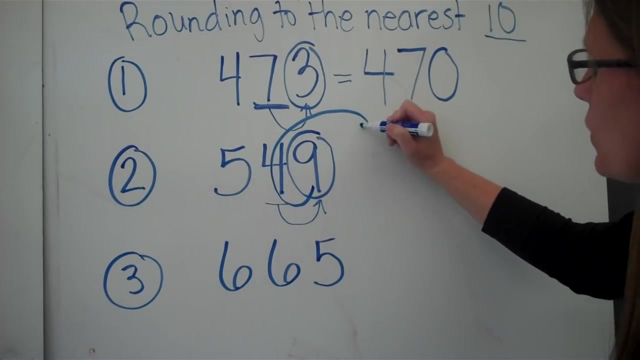 at number two. Again, I'm rounding to the nearest tens, so I'm looking in the tens place And then I go one column to the right, which ends up being my ones. Nine is a strong number. it pushes the four up to a five. This nine becomes a zero, and then I'm going to write. 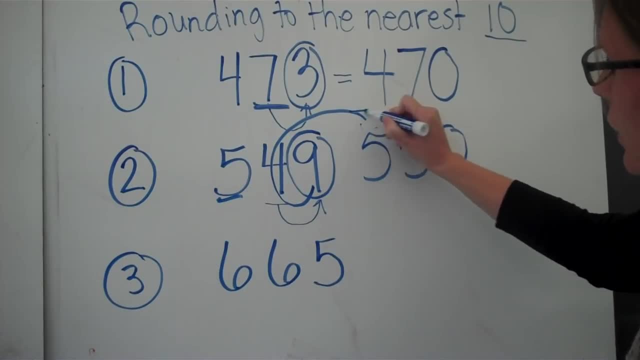 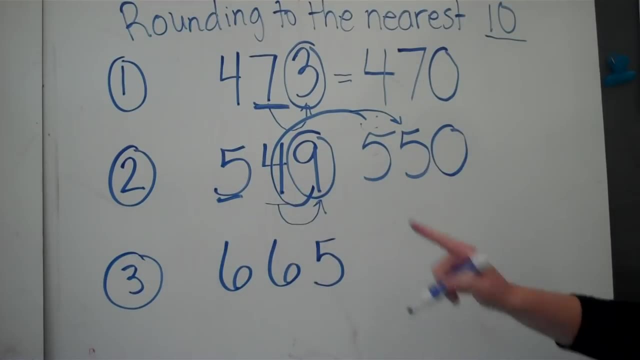 in my hundred. This arrow should really be going over there. So 400, or, excuse me, 549 rounds to 570.. Again, I'm not looking at the hundreds, so the hundreds are just going to stay the same. Next one, looking at nearest ten: go one column to the right. I have a five. Five is nice.